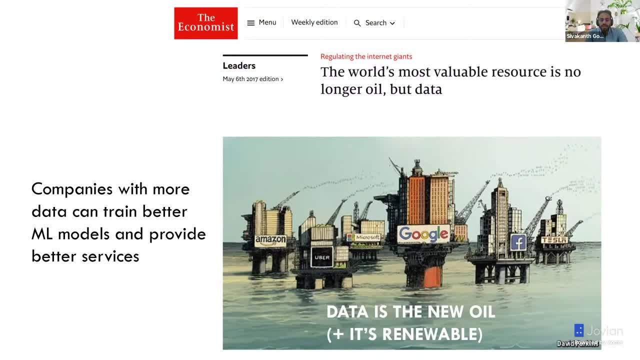 Because, especially now in there, when AI models are getting better and better, you know the difference between companies ultimately might boil down to like the quality of the data that they have Right. So there are all these scaling laws for neural networks which show that to get better and better, you need more data. It's not just compute, but you also need more data. So you need both compute and data to get even better. 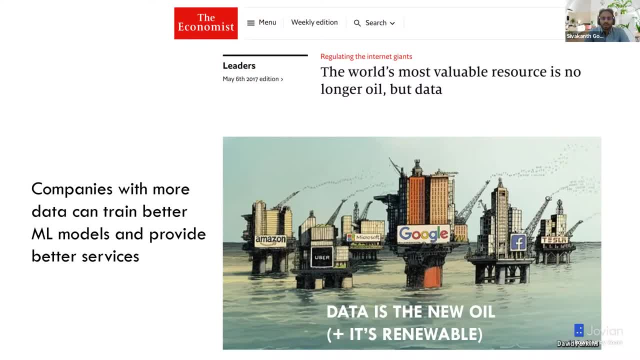 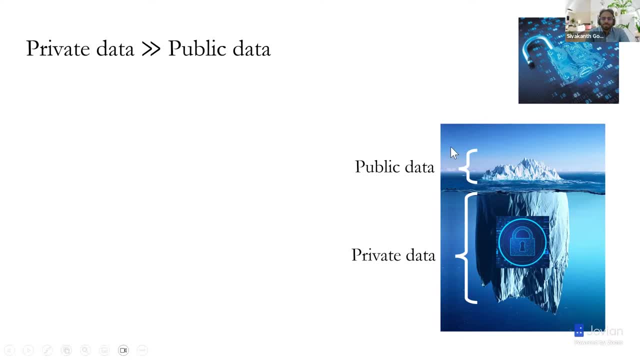 So you know data is really important. The only issue is that a lot of this data is private, So you know. so if you think of the public data, which is what we see publicly, that everybody sees on the internet, it's the tip of the iceberg. 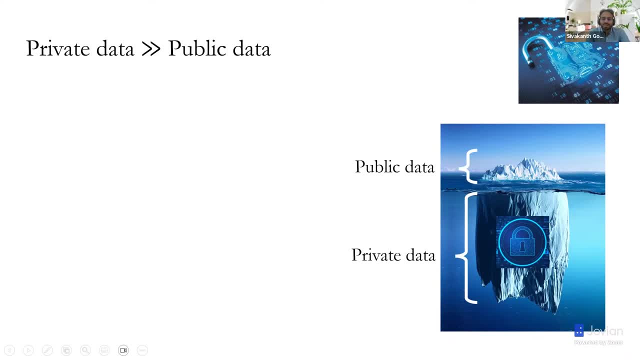 There's a lot more underneath which is private And on that, Only these big companies have access to. So this and it's a lot of data, because I know that, I know I know this because I'm at Microsoft and I see you know huge amounts of data. 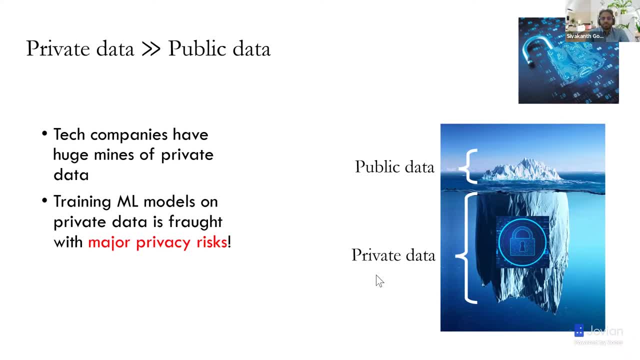 They have never charted on data, But the only issue for them- for most companies, is that this is private data and it's sensitive. So if you train a machine learning model on this private data and you release this model to do things you know other things, there are major privacy risks. 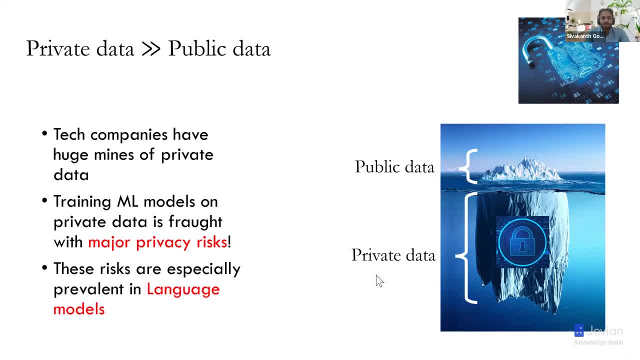 And I'll talk about you know what these risks Are in a bit. And these risks are especially prevalent in large language models because, you know, these are generative models and they have this issue that they memorize verbatim, whatever sometimes some of the training data they're trained on. 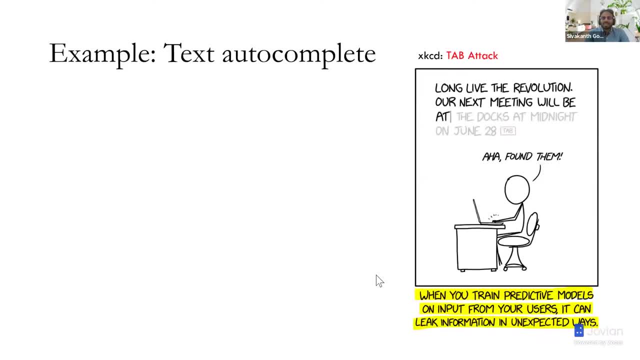 So here is a fun example of like what can happen if your model memorizes a training example. So XKCD has this comic where you know a cop is trying to find some revolutionary Is for like plotting against the government and what you know all the revolutionaries are, you know, communicating by email. 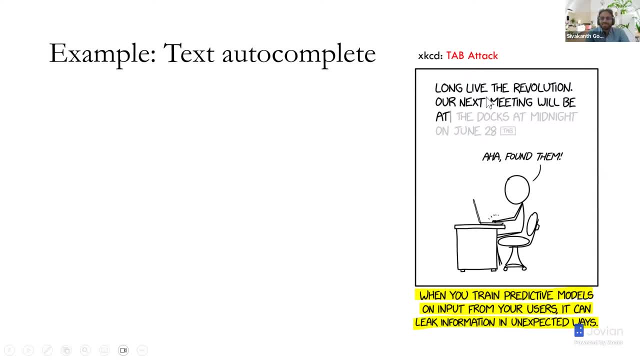 So what he does? and you know, Gmail trains their models, their autocomplete models on personal emails. So the cop is just like. long live the revolution Our next meeting will be at. and then you know, he just presses tab to autocomplete. 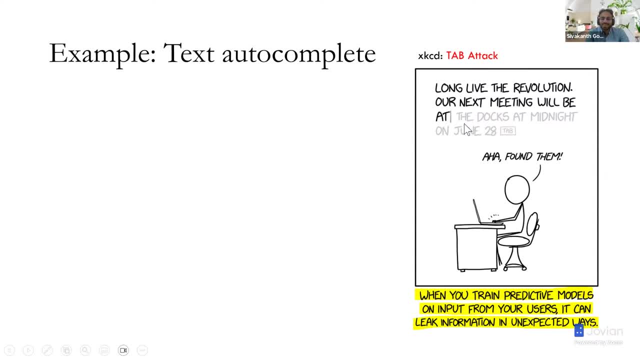 And then the Gmail client or any other email client is just autocompletes to. we are meeting at the docks at midnight on June 28th, So this is Sort of things that that we want to prevent. that you know, when you train this predictive models on, you know personal data- there is such a chance. 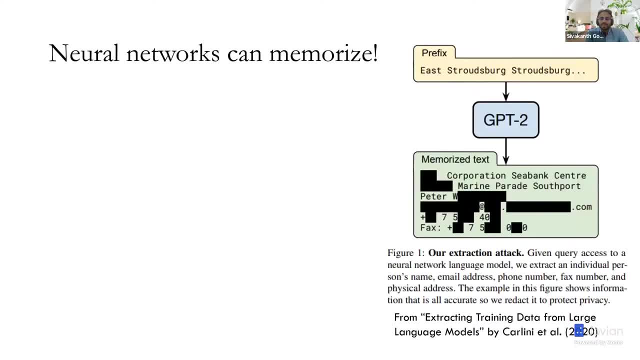 And this is not just a comic. This actually happens in practice And people wrote papers. So there is this famous, famous paper- because any at all- it's called the secret share paper, where they took this GPT-2 model, which is a large language model trained by open AI. 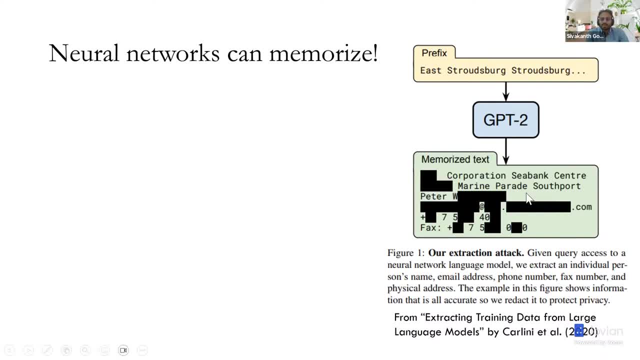 And then they extracted a lot of you know, private information from it, Like in this case. like you know, you Can get emails and phone numbers and whatnot of different kinds of people which is not supposed to be there. 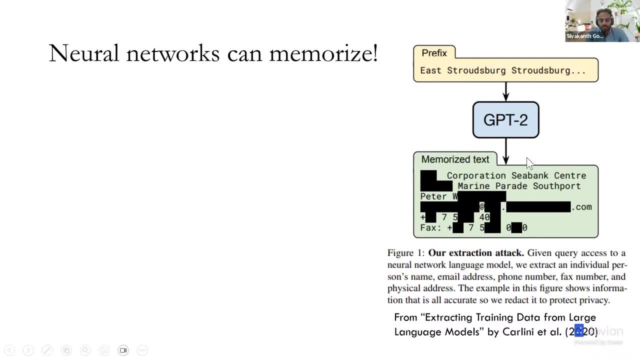 And this is just an example. But you know, technically GPT-2 was trained on things on the Internet. But if you do the same thing with email data, then you know the same thing can happen. Like you know, your bank account numbers and credit card numbers can come up here if you prompt GPT-2. 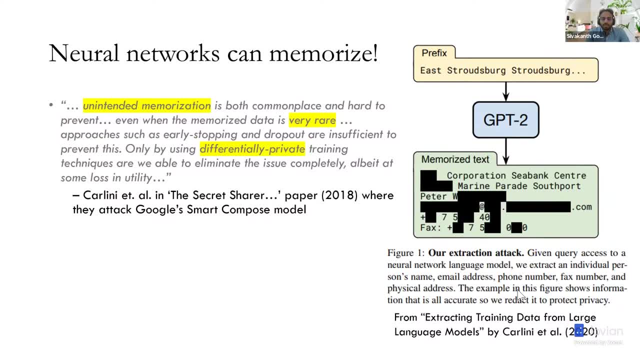 So. so these are the sorts of issues that we see, And- and this paper which did this attacks- also showed that there are lots of Ad hoc ways to kind of stop this and all this, ad hoc privacy mitigation measures, but not really working. 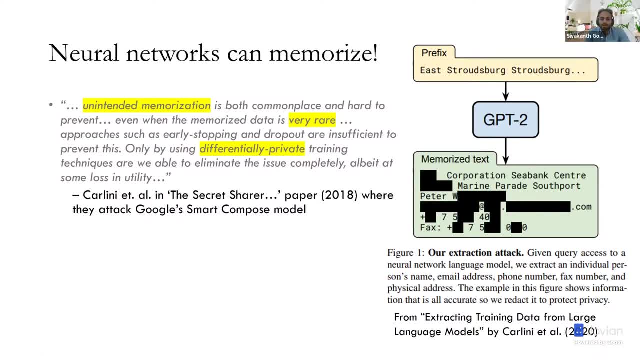 And what really worked is this technique called differential private training and which, you know, though it's not perfect, but that seems like the best mitigation measure that we have to stop this kind of stuff. What does this differential privacy mean? And the rest is like optional. 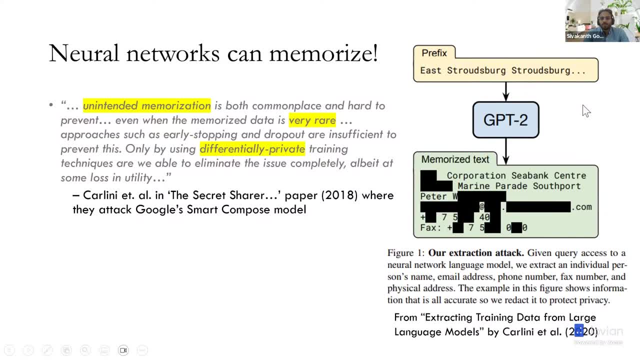 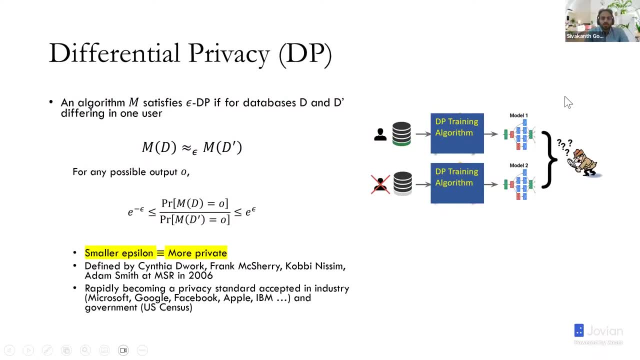 OK, so what is this differential privacy? So I'll spend a bit of time on the definition, because I think That's the most important thing that most people should know: It's that. so if you have an algorithm, so so let's say it's a training algorithm, it's a machine learning model which takes some data and then outputs a model. 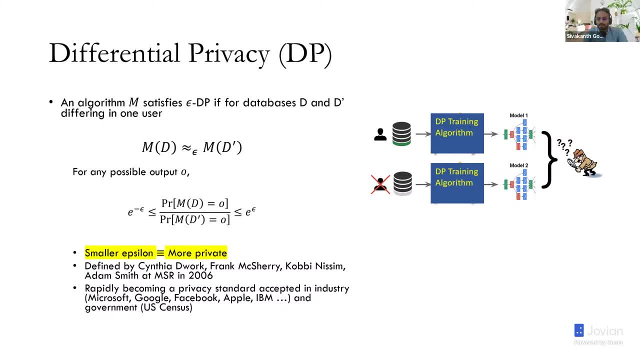 So my algorithm is not the model itself, It's the training algorithm Like, for example- it can be SGD, stochastic gradient, descent or some other learning algorithm, convex optimization, some learning algorithm which looks at user data and outputs a model or some other output. 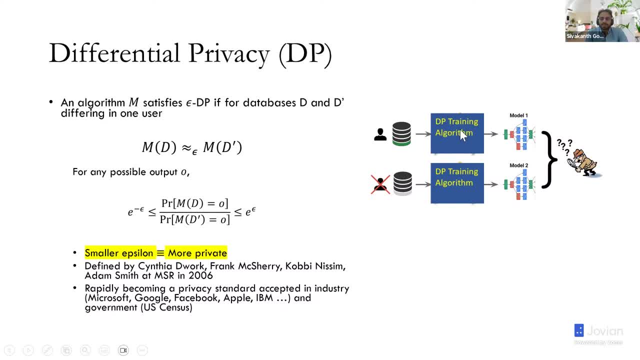 So and this algorithm? Let's say it is a randomized algorithm, which means it's not always producing something fixed. So we say that this algorithm is epsilon differentially private if on neighboring databases, which by which I mean that take a database and you change only one user's data in this, in this database. 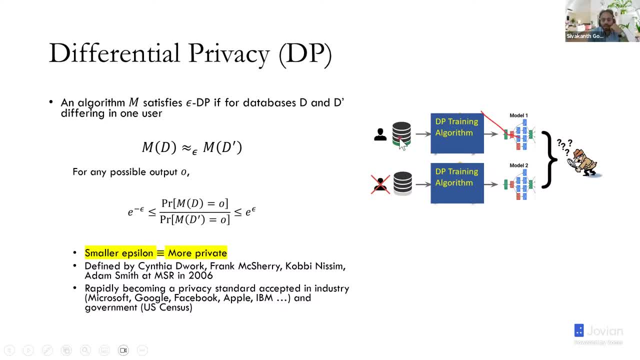 So so here I don't know, maybe it is- And then you imagine it's a thought experiment where you imagine training it on two edges and databases which only differ in a single user's record. So, like Here, You can see that a single user's email was there in the input and here there's single. that user's email is not used during training. 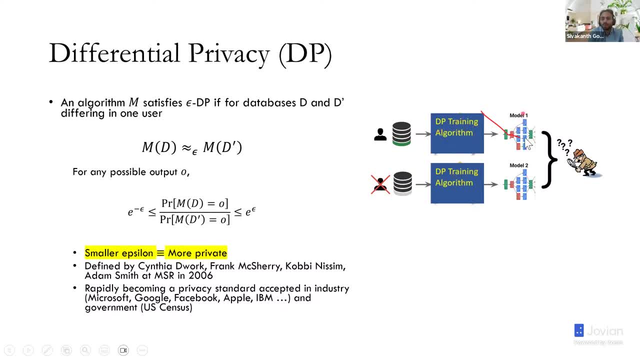 And then this training algorithm produces two models, or model one and model two. And now, and you're given an adversary access to these, to the models, you know they can do inference, they can even look at the weights and they can do all sorts of things. 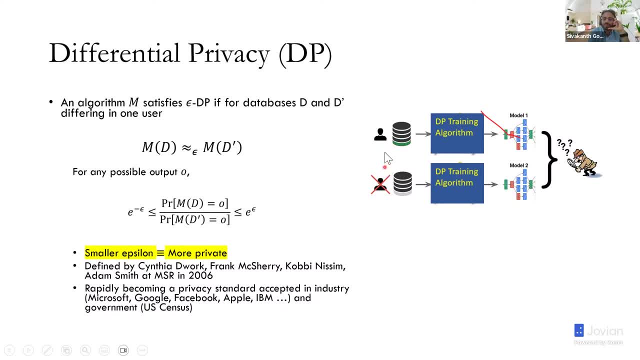 But then they were trying to find whether this particular user's email was used or not used. So they want to distinguish between these two cases. whether you know, I give you one of these models, these models at random, to this adversary. they can't tell whether it was trained with this user's. 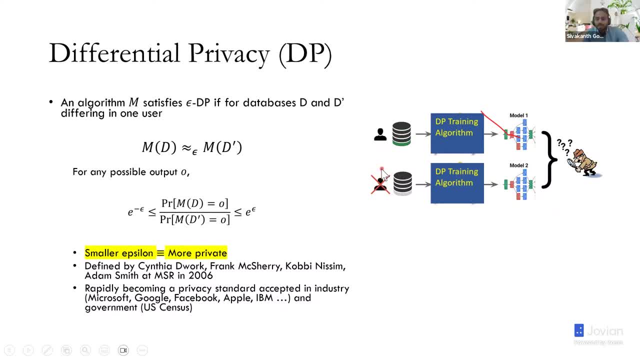 email or not. This is a very strong privacy protection, which means that if you can't even tell if the user's email was used in the training, it means that no personal information of this user can be there inside the model's weights or during its inference, and so on. So that is the definition. 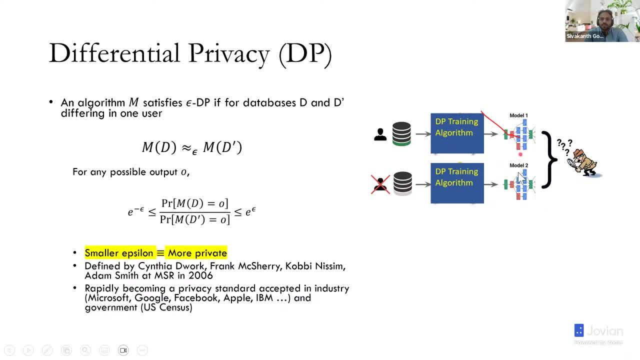 So, more formally, how do you say that these two models are hard to distinguish? So, as I said, this training algorithm is a randomized algorithm. What it means is that what it outputs is not a deterministic single model. It outputs a distribution of models And in general we say: 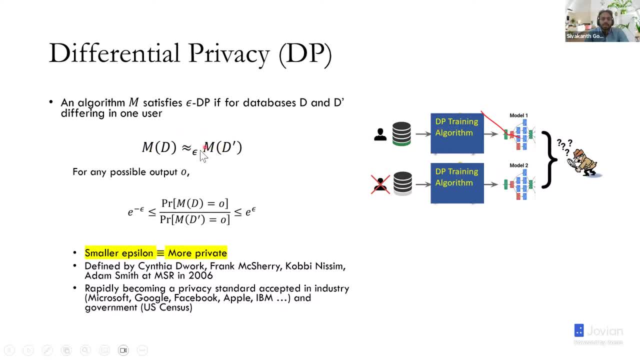 that such an algorithm is epsilon differentially private if the distributions are epsilon close, by which I mean that if you take the ratio of probabilities that it outputs any particular model, the probabilities of the ratios is bounded by some constant e to the epsilon and lower. 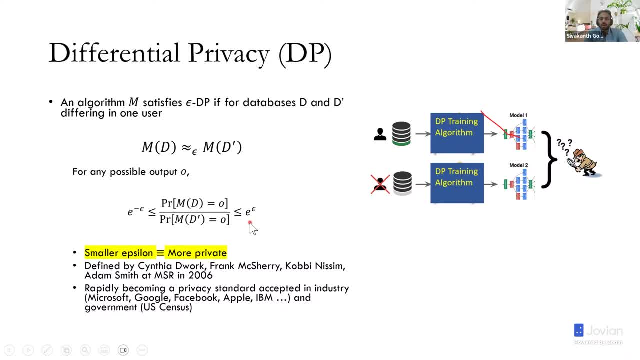 bounded by e to the minus epsilon. So it's a measure of how close the probability distributions are. We're saying that on adjacent databases the algorithm outputs very similar distribution of outputs And obviously the smaller the epsilon, the more private the algorithm is, which means that if epsilon is like 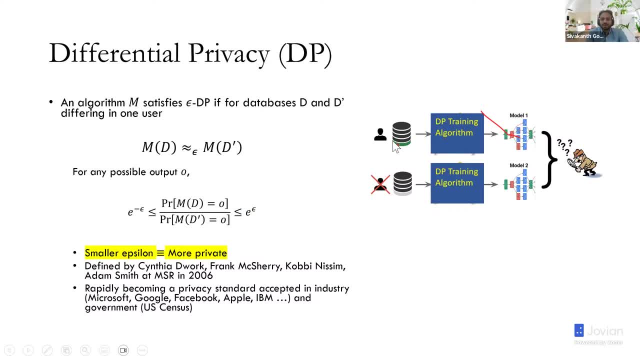 zero. that means it's perfectly private. It's not even you know. it doesn't matter whether this user's input is there or not. It's outputting the same distribution of models And the smaller the epsilon, the more private you are, And this definition has been introduced. 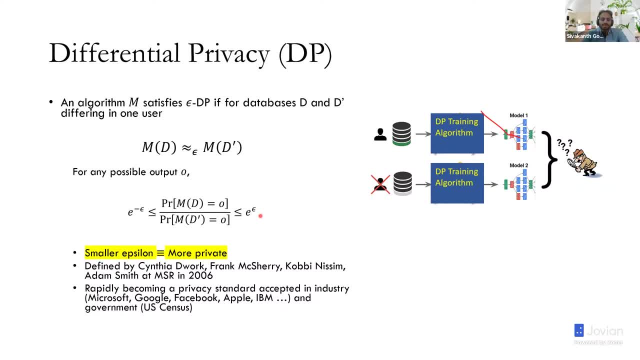 in theory in like 2006.. And since then it's been increasingly adopted, you know, in industry like Microsoft, Google, Facebook, Apple, IBM. They, whenever they, you know, train models on private data. they also include that you know they do it using differential privacy and they 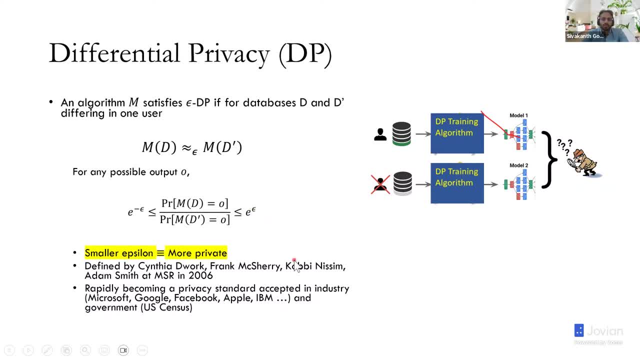 tell you, oh, it is, we trained it with so-and-so, like epsilon equal to one, epsilon equal to two: differential privacy. Moreover, the US government also believes in this technology. So the latest census in India, though, they didn't have it, you know, for the past three years, but it's that. 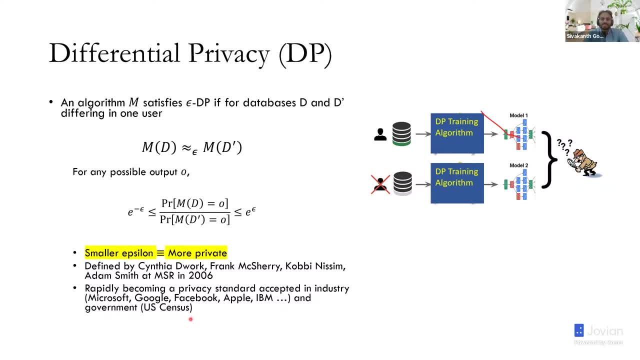 every 10 years they do a census in US as well. This- all the census data- has been released using differential privacy because they also felt that the US government felt that there was lots of privacy risks. If I just if- they just announced the census data without, without any privacy. 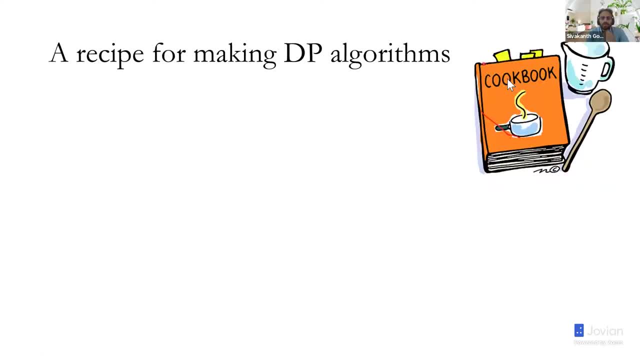 mitigation measures. So so let me tell you a little. you know recipe for how do you make you know a differential privacy measure. So let me tell you a little. you know recipe for how do you make you know a differential privacy measure. So let me tell you a little, you know. 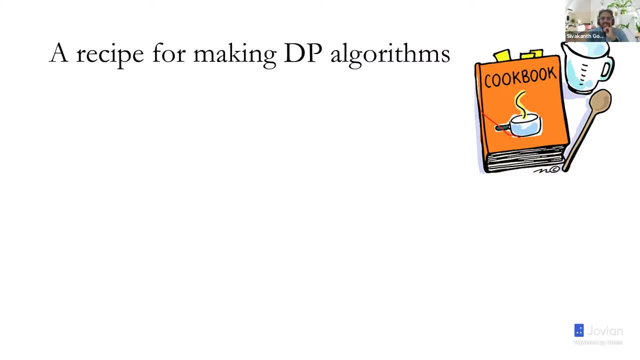 sort of a cookbook for DP algorithms. So it's actually pretty simple, like for. okay, there are complicated algorithms, but in most use cases the algorithm is very simple, So it's a very simple recipe. So first you limit, use individual user contributions to some small 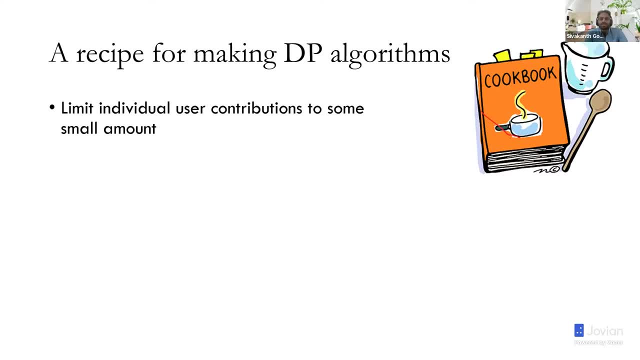 amount. You kind of say that nobody should try to influence my algorithm too much. So you, you try to limit it in some way, And then the really key part is need to use add noise to individual user contributions without adding noise. So you kind of say that nobody should try to. 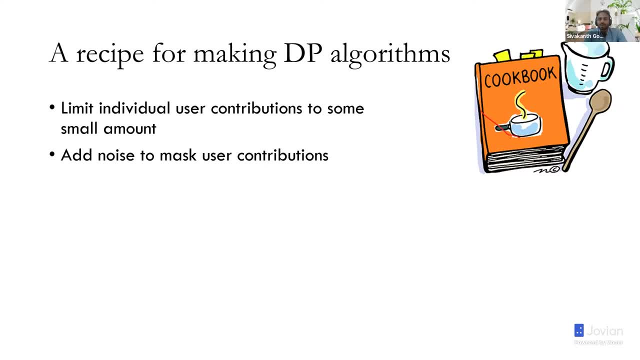 influence my algorithm too much. So you kind of say that nobody should try to influence my algorithm. without adding noise, You can never make anything different to private. As I said, if your algorithm has to be randomized, it has to introduce some stochasticity, some noise into the process to mask. 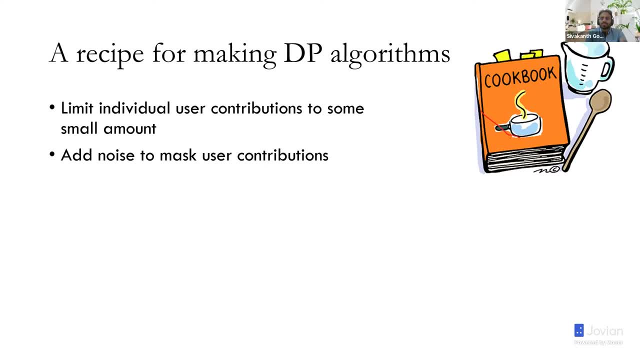 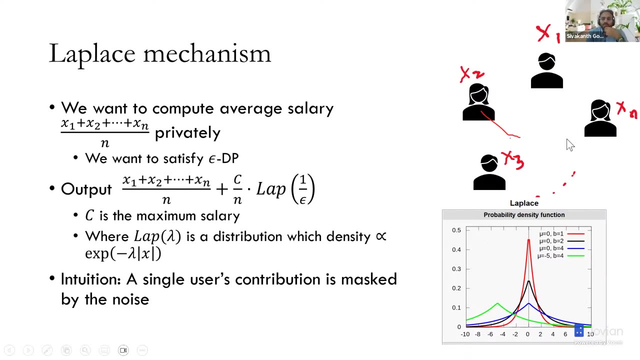 the process to mask the individual user contributions. So this is, these are the two main steps, and and this, this, that's it. So you limit user contributions, add noise. So let me give you an example of how this recipe works. Let's say I have a simple problem: I have N people in a room. 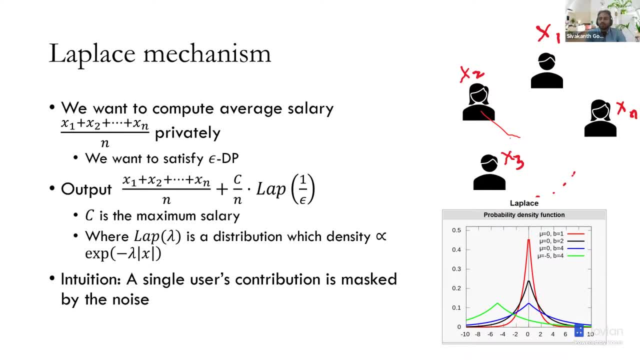 and they want to compute their average salary. And I want to compute their average salary And I want them to compute that in a private way, So nobody wants to reveal their, like you know, their, their personal salary, And and let's, and let's assume that they have like a trusted party who they 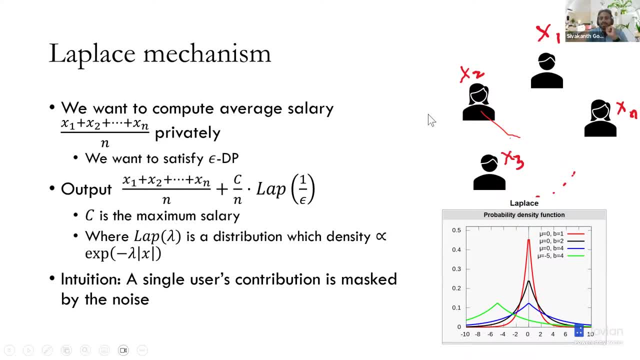 trust so they can communicate the whole thing. All they want to know is that average salary of everyone. Okay, So what differential? and we want to do this using differential privacy. So what differential privacy does is like you just compute an average and then you add some noise And then 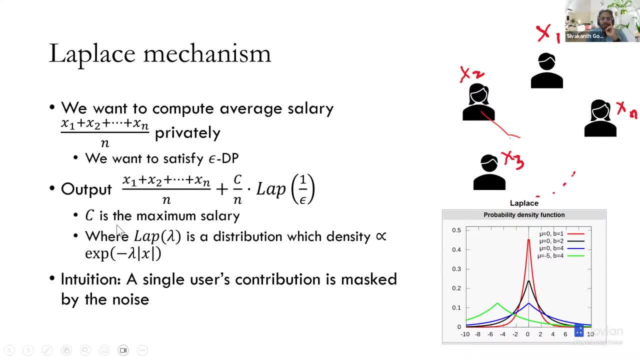 you also assume that you know each salary is bounded by some amount. let's say C. So C is the is the maximum salary. nobody's earning more than like, let's say, one crore per annum, and so that is your c and, and then if somebody is earning more, you just truncate. so let's say the. you know there's. 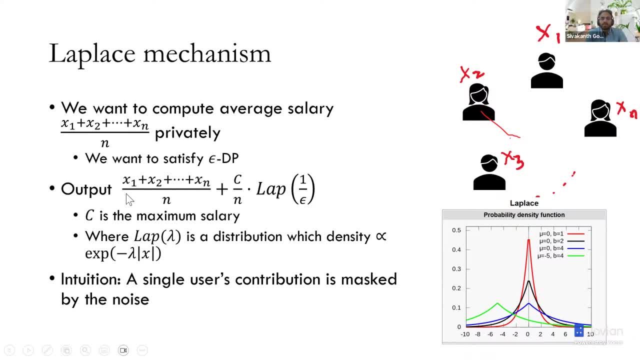 these are anomalous people. so you just truncate and then you just assume that everybody's have bounded salaries between zero and one crore and and then you just average and you add noise which is proportional to, uh, something called lap. it's called a laplace noise, so this is a particular 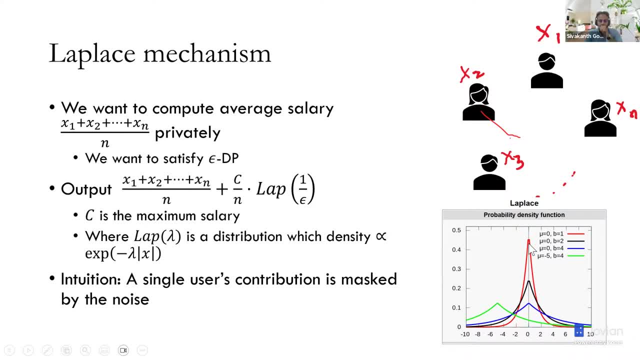 noise distribution which comes up, you know, which is specific to this, uh, differential privacy. so, yeah, it has a particular density. its density is like exponential in minus, uh, lambda times, the absolute value of x. and on the right you can see a picture of how this distribution looks. it looks like, you know, it has a peak at zero, so it's a not so basically you're. 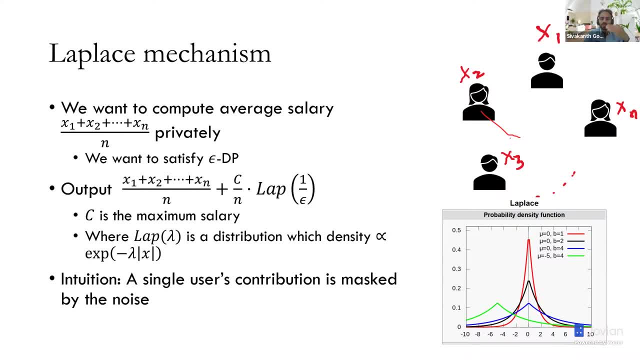 just computing the true average. you first look at the average and then you look at the average, and then you look at the average. you limit the use of contributions, compute the true average and add a little bit of noise. so now this noise makes it really hard for me to distinguish whether a particular you know find a. 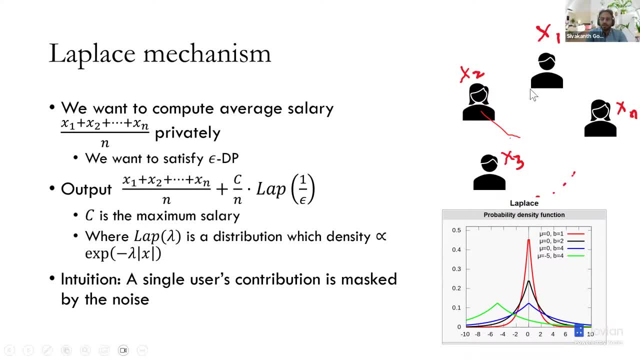 particular user's salary. why is that? because even if i know everybody else's salary- let's say i know the salary of everyone except x1- i still. so what i? what will i then know, is x1 plus x1 over n, plus c over n times some laplace noise. i can multiply it by n, so what i know is x1 plus laplace noise. 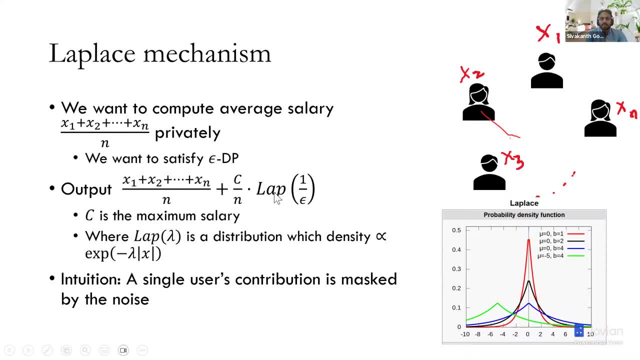 right, it's like and and then i'm adding, i'm multiplying the laplace noise also by c. it means that even if this user salary is zero or c, i cannot distinguish because i'm adding noise which is proportional to the maximum amount c. it's like if you have one noisy sample. 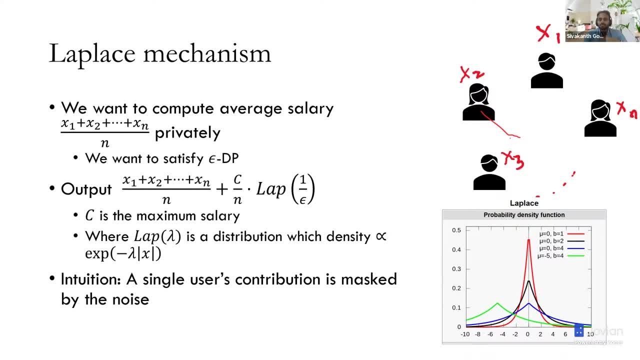 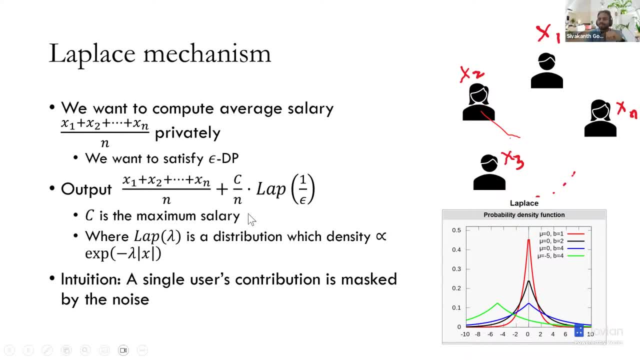 intuition why it works and you can prove mathematically this satisfies the definition i showed you. and- and that's where this particular distribution of noise comes in- because i want the ratio of probabilities to be bounded absolutely by a to the epsilon. this particular probability density will do that, do the trick for me, it's okay. but the intuition is that you're just masking an. 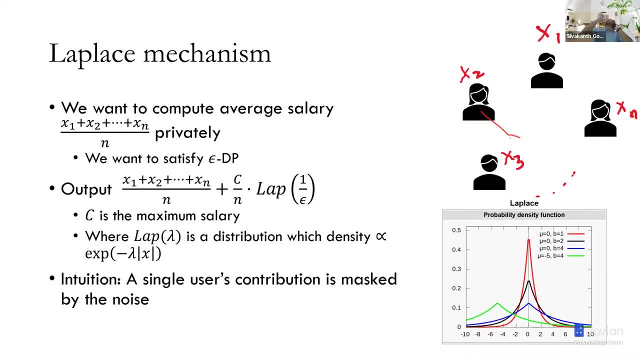 individual user's contribution by noise and- and the good thing here is that see that the noise scale also scales like one over n times, some, some constant amount of noise, which means that if there are many, many users, the amount of noise that i need to add to make it private also goes down to. 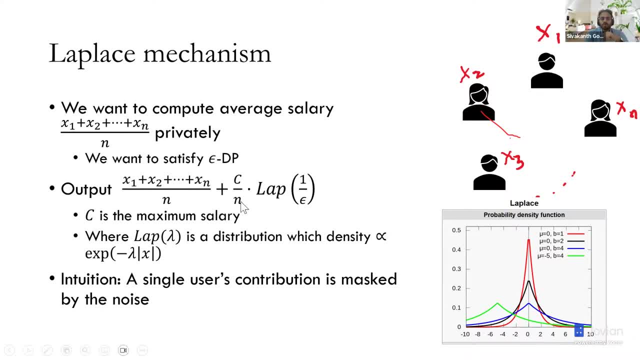 zero. so as there are more and more users, i'll get more and more accurate estimate of the true average salary, but at the same time, i'm i'm preserving everybody's privacy. okay, so this is the general story with privacy. as you can have more and more users, you can give them more and more privacy, as. 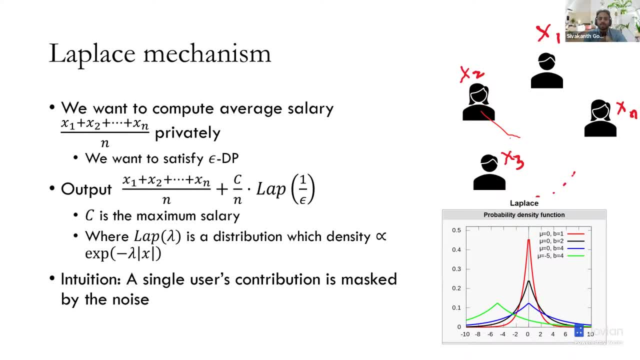 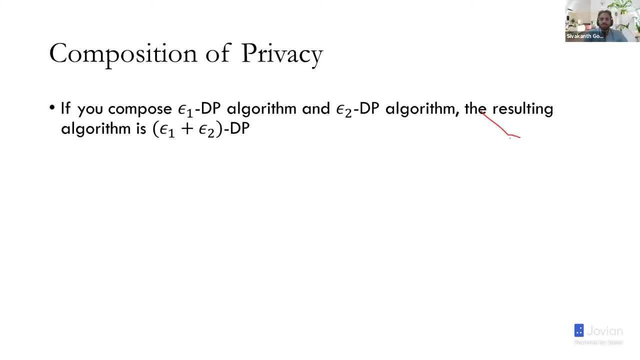 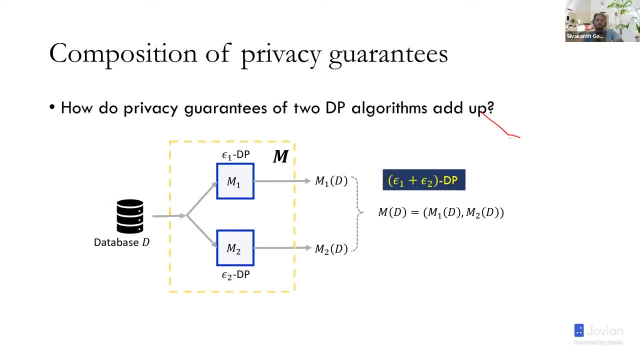 well and at the same time, learn a general statistic or general trend more and more accurately. okay, so that? so the other good thing about differential private algorithms is that they compose very well. so if you, you first- uh, you know, i think i have a picture- it's better. so if you, you. 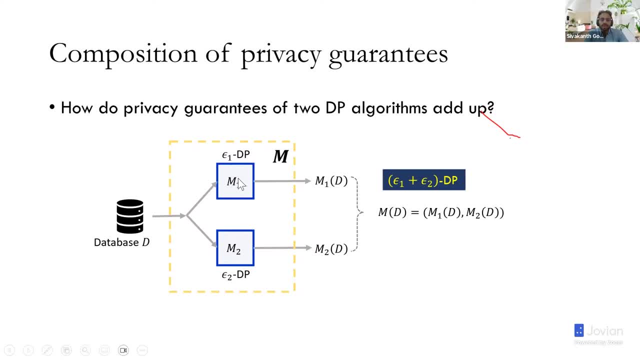 have a database and you have a machine learning algorithm and you train a mission model and you output it. and the first algorithm is epsilon 1- dp, and the second one you, you, you do it again. and then the second one is epsilon 2 to dp. the together, the total privacy loss you you will face, is just 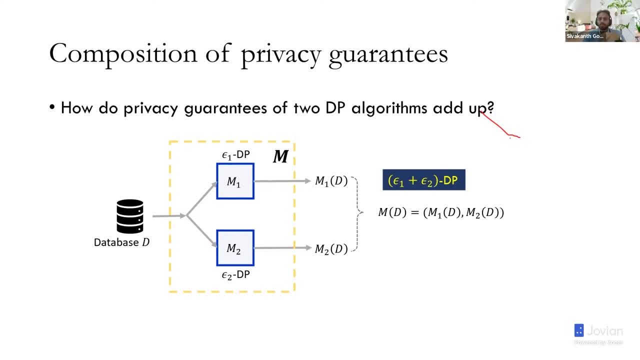 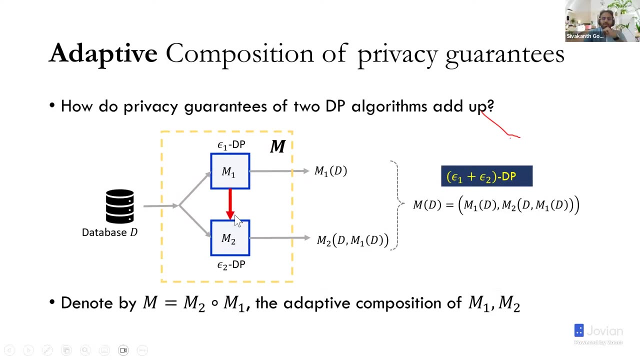 the sum of the epsilons. so this is a nice property of uh of privacy. you know this, this differential privacy, that if you keep releasing information about a database using differential private algorithms, the privacy loss that you incur just adds up. moreover, this you can do it even. 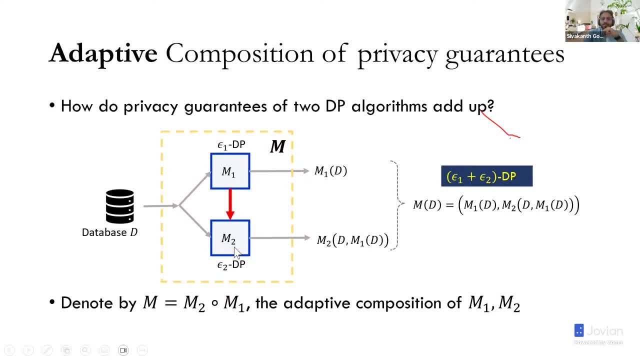 adaptively, which means that the second algorithm can even look at the output of the first algorithm and then output and then do something with it. And still, if the first and second are individually differentially private, the whole process is differentially private, And this is one of the nicest thing. 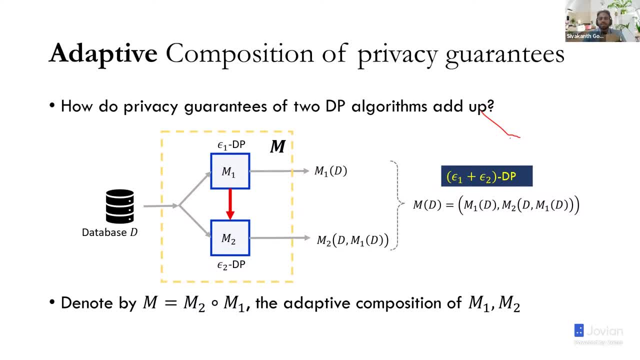 about differential privacy, because in general, this is what happens. It's not like you just train it once and it's over. You have lots of private data. You keep doing things with it. You train one model, You train another model. 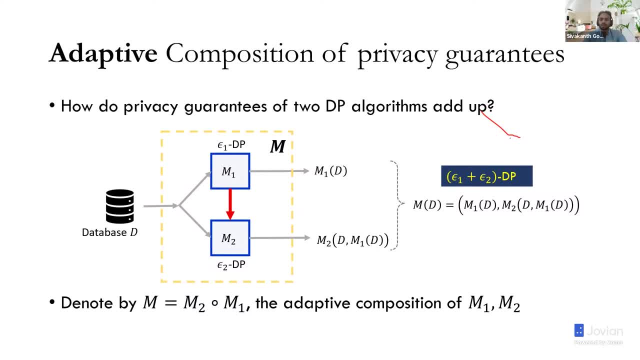 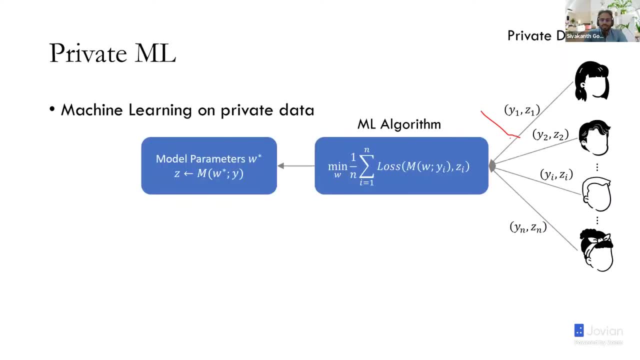 You learn something, You learn more things, So you want to understand how the total privacy loss is happening as you do the training more and more. OK, so now let's talk about the specific context of private ML. So, Aakash, how much time do we have left? 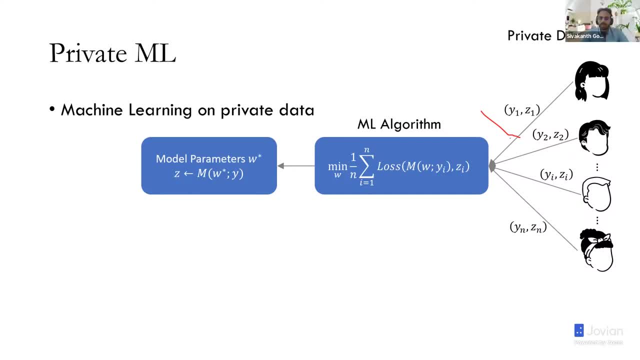 Yeah, I think we have about 15 minutes. OK, great. So let's talk about private ML. So what we want to do is: what do you expect? So each user is giving some example, Like let's say, you know, let's take the example of, maybe, ads. 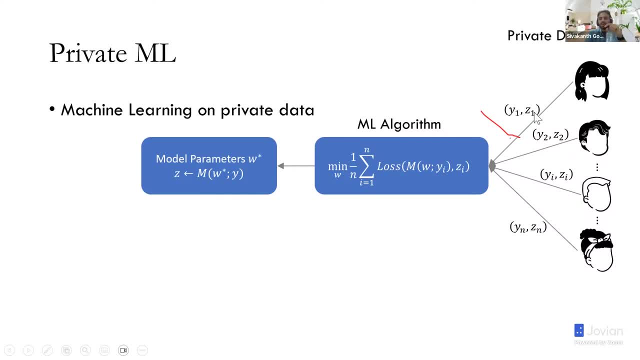 So each person you show them some ad and they click it or not. they don't click it. You can think of it as an easy and why is the ad you show them? and things like that. So this is the private information. or it can be like why one is an email that they wrote and Z1 is like whether 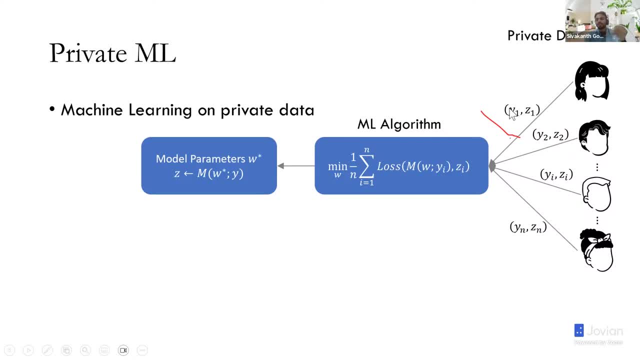 you know, or Z1 is the next word, So Y1 is like the prefix and Z1 is the next word in an email that they train. And then you want to train a machine learning algorithm which predicts Z given Y right. So this is the standard thing. but here now you're assuming that each user is 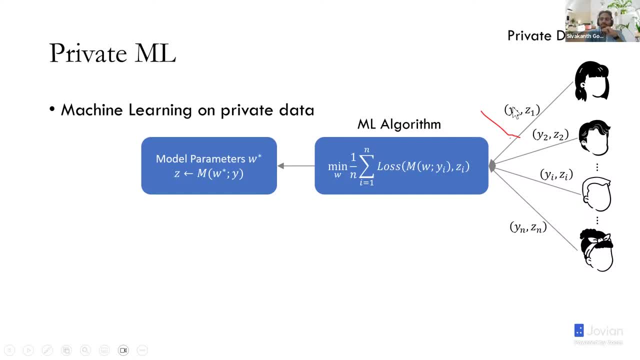 is. you know this, this input that you get from each user is a private information and you want to protect this privacy of this users And this is the general trend. Like you know, this is how all these tech companies collect data. 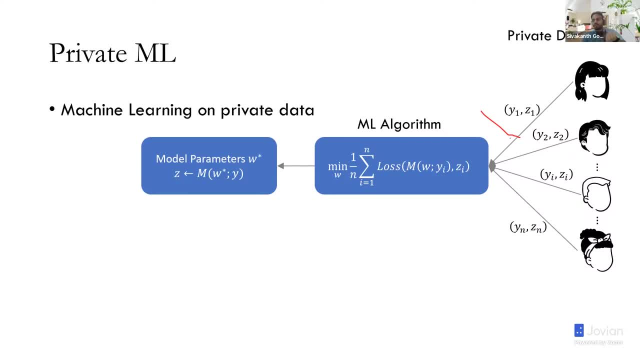 They collect small, small amounts of data for from millions and billions of users, And then they want to train a machine learning model which fits all this data that they're collecting, And then they want to train a machine learning model which fits all this data. 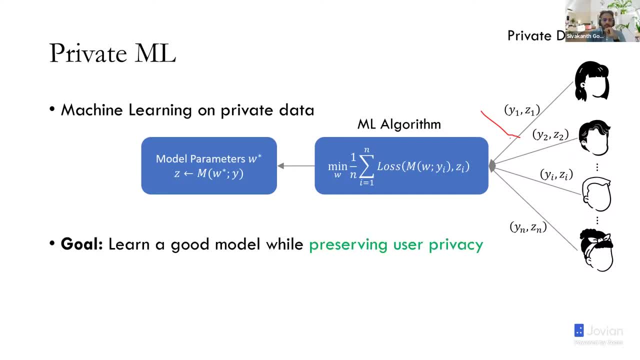 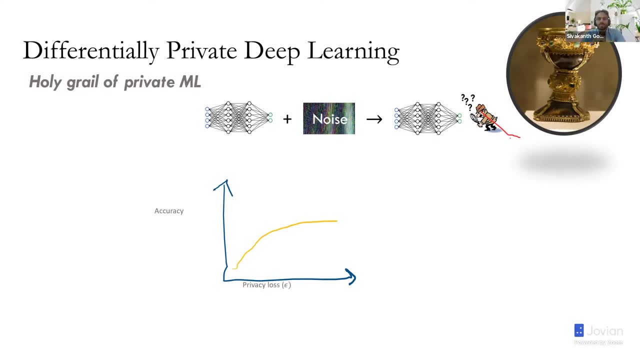 they observe across all these users. So so learn a good model. Okay, So specifically, you know machine learning models. the most common ones are, of course, deep learning models, because that is, you know how, where the world is heading. You know we want to train deep learning models using 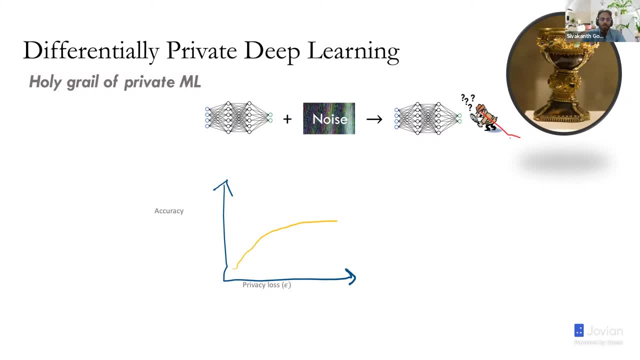 differential privacy as well, And that is like the biggest question, open question in this whole area of differential privacy, Like how do you do differentially private deep learning? So we want to add, you know, as I said, the goal is to add some noise, you know, to the weights. 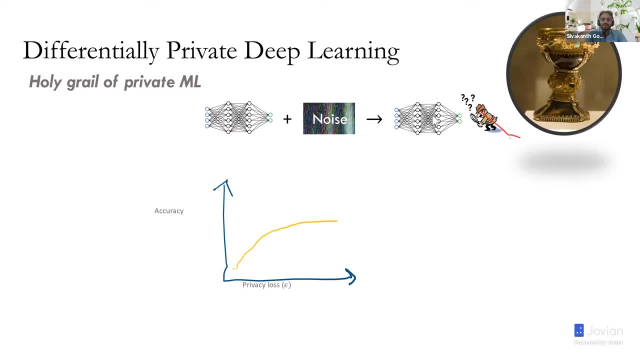 you know in some controlled way so that you can. the adversary, can you know- cannot tell anything about the data that it was trained on by looking at the model. Like, in particular, you can't tell whether particular users data was used or not used by looking at the model. 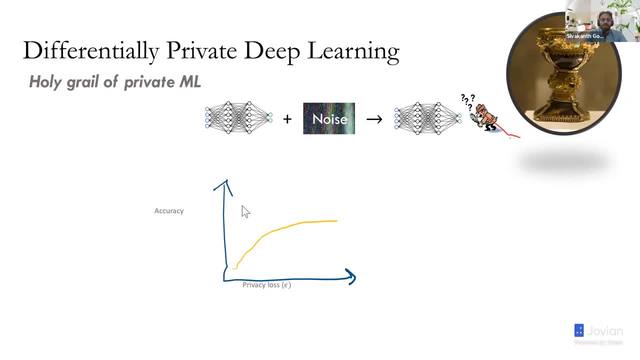 And in general there's a cost to privacy. Privacy doesn't come for free. So you know, if you plot the accuracy versus the privacy loss, then it's. you know, the more privacy loss you can incur, the more accurate it becomes. So this is called the, you know, the privacy utility trade-off. So 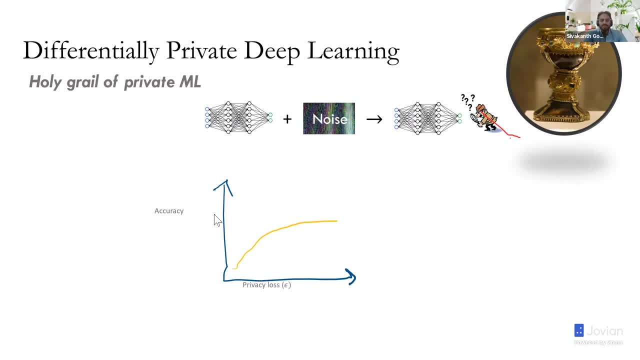 it's like if you want to be really private, you have to face some loss in accuracy. But if you're okay with losing a little bit privacy, you can get more and more accuracy And, like as epsilon tends to infinity, you get the non-private accuracy which is like when you train a non-private 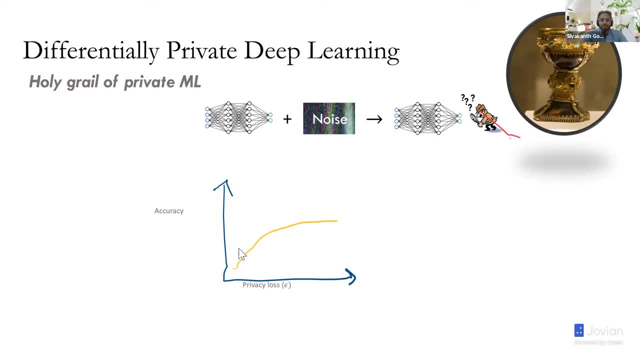 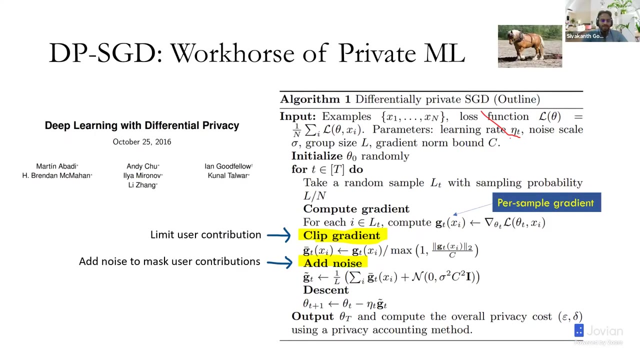 machine learning model on the same data, that's the epsilon, equal to infinity. So you know, there is this trade-off And the goal of this whole area is to, you know, make this go higher and higher. So, okay, so let me show you. you know, this is the only promise, that this is the most technical. 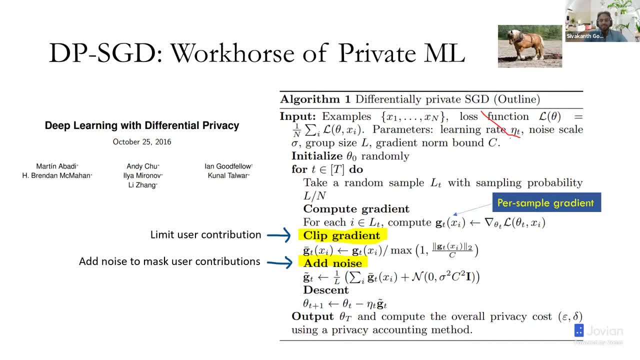 slide of the stock, which is you know how to actually make the you know training of different deep learning models differentially private. I so I yeah, at least for the slide. I'm going to assume that you know how machine learning models are trained without privacy, which is this algorithm. 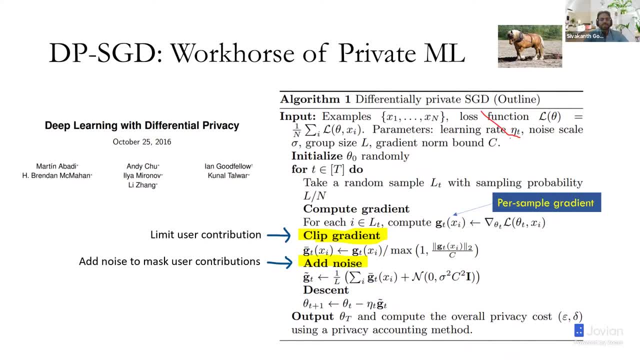 called stochastic gradient descent and some variations of it, like Adam and whatnot. But but the basic algorithm you know. I hope that you you know this, which is that you have many examples and you want to minimize the loss function, which is the average of the loss over. 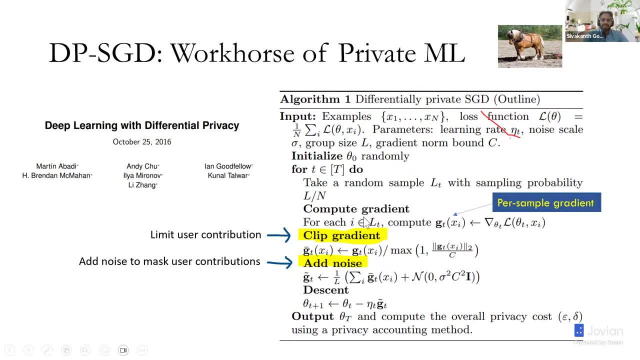 all these examples. So what you do in STD is you you sample a random batch from this set of examples and then you calculate the average gradient. So the gradients of the loss function with respect to all the samples and the average, this gradient. 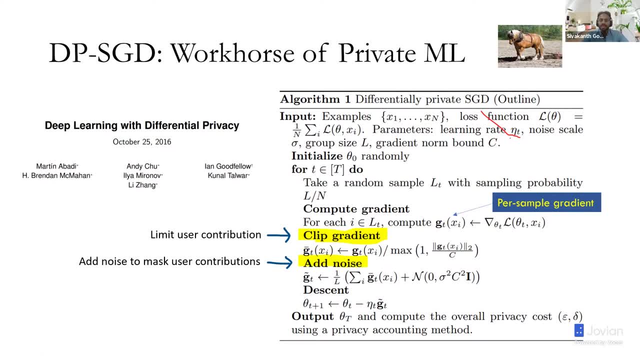 uh, gradients, and you get the average gradient across this batch and then you take a descent step in the direction of this average gradient, right, And then so you update the weights, you, you, you do a gradient descent step. So this is the usual STD. So now we want to make it private. 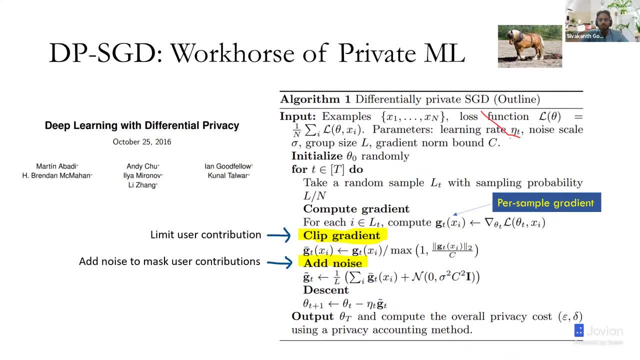 and and we are going to use the recipe that I showed you, which is that you first have to use uh- limit user contributions- and then you need to add noise to mask user contributions. So, because each gradient is computed on a particular user sample. 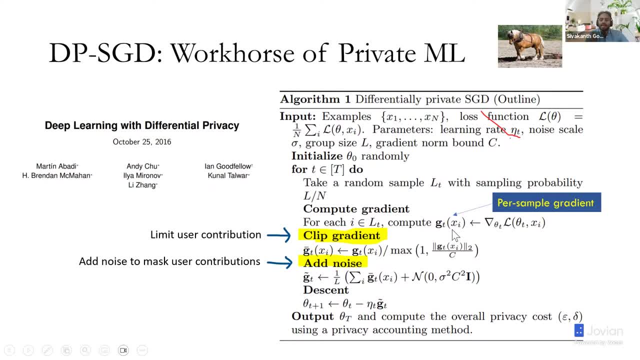 it means that this is private information, Like the gradient is telling you some private information about this user, So you need to limit the user's contribution. So what we will do is we'll clip the norm of the gradient to some constant C. So if the norm is too big, it means 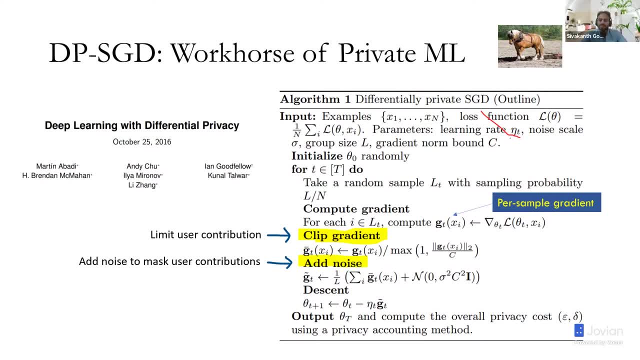 that you know we are getting too much information from this user and we don't want to use all this information. So we clip it to have norm at most C. So this is the clip gradient step. So you, for each gradient, you clip it to norm at most C. And then we do the Laplace mechanism, which is you: 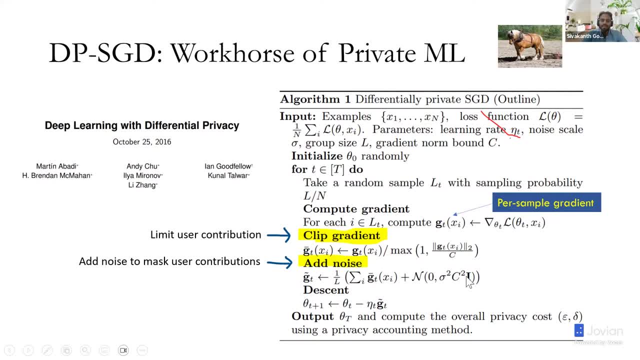 to the average gradients, you're going to add some noise, And in this case I'm going to add a Gaussian noise. So, and then I do the gradient descent step. So it's pretty simple If you think about it. this is exactly the recipe I showed you. You just clip the user contributions and then add. 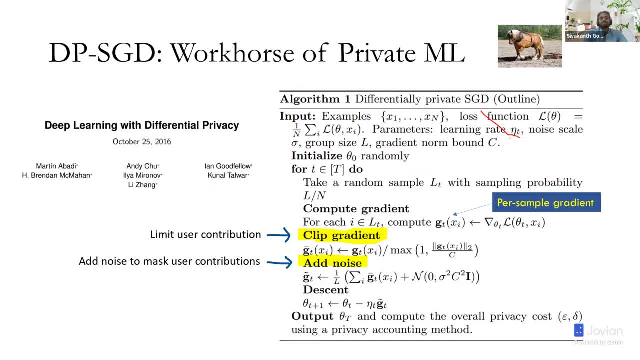 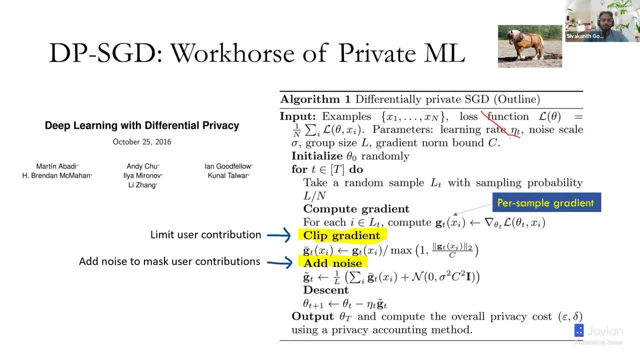 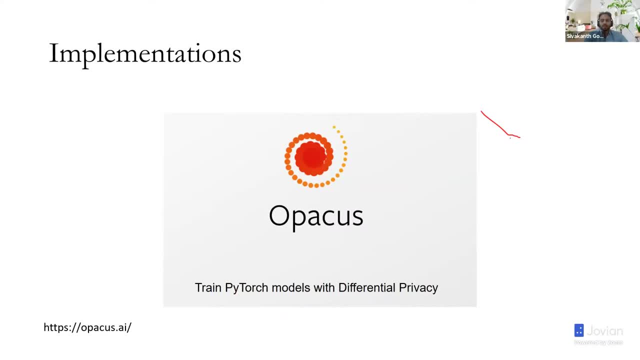 uh, but it's a pretty simple algorithm and you can prove that it is differentially private And and there are already implementations of it. Like you know, if you, there is a pretty standard library called Opacus, which you know which was, which is built on PyTorch, which allows you to 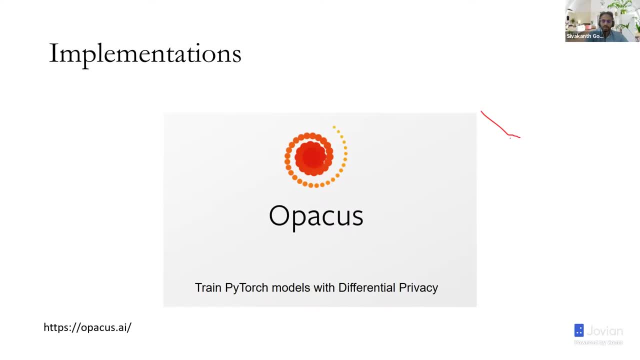 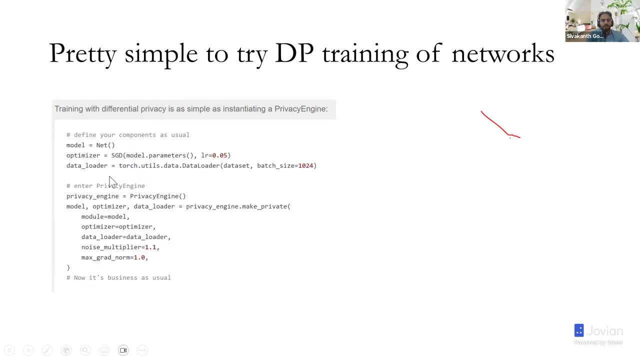 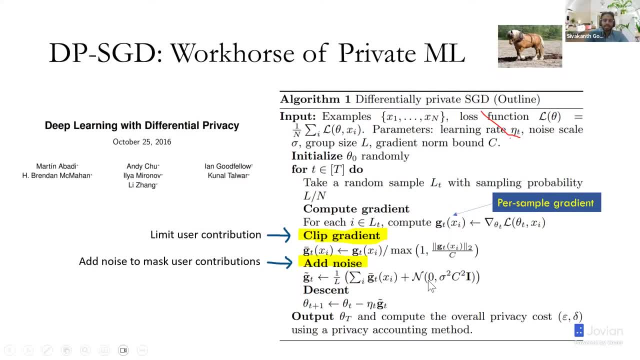 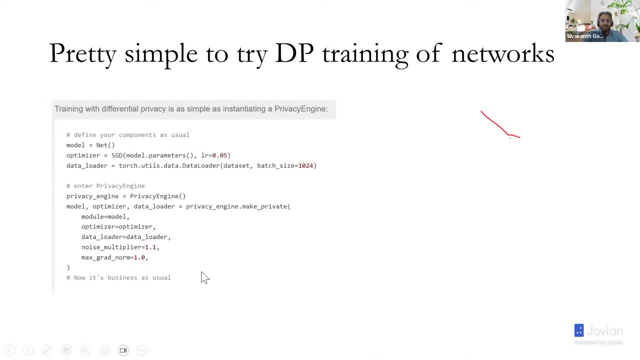 hyper parameters Like, for example, what is the noise, that Sigma that I need to add here? What is the clipping norm, How, how small should I clip my norms? And so on. Once you give these things it'll, it'll output the epsilon, the differentially private parameter that your 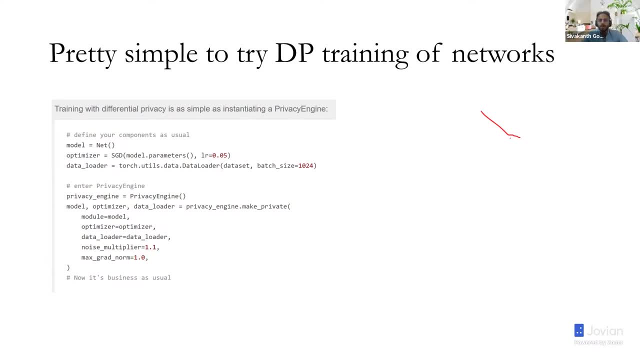 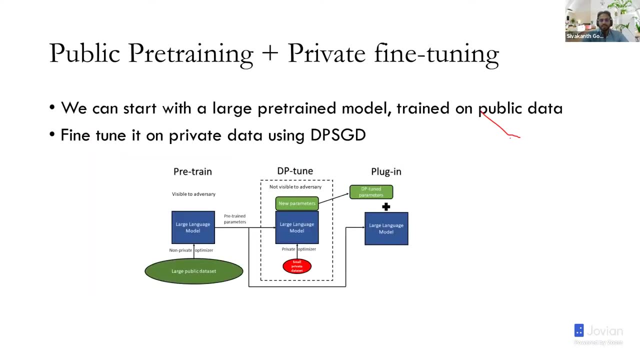 algorithm is: uh, satisfies, And I will also give you the final model that is trained, So you can try it out and and it works pretty well in practice. So, and one more trick that you can do is, like you know, we don't need to, uh, you know, find, uh, train our model. Let's say you want to. 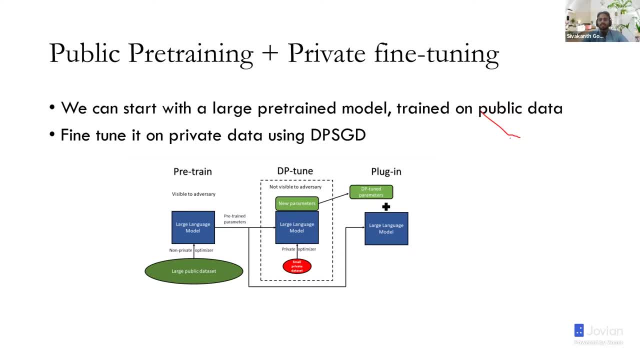 train our model on private data. but then if you just start from scratch- you know you, you initiated your model ran with random weights and then you start training- It doesn't do too well. Like you, you take a big hit in privacy. It's a big hit in accuracy because of the, because. 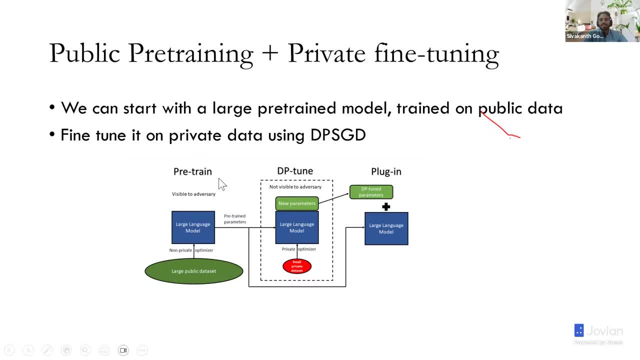 we're imposing privacy. But what happens is, especially now we have this huge pre-trained models- Like if you go to hugging phase, you can download like thousands of uh, uh, uh, uh, uh uh, thousands of thousands of pre-trained models which are really good and trained on large. 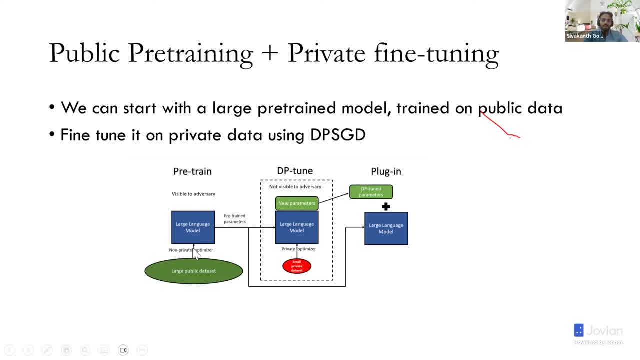 amounts of data. You start with this model and you assume that it's trained on public data, And now you can use DPS city to fine tune it on your private data, which is very small. And then now you output your new model, which is which is like fine-tuned on private data. 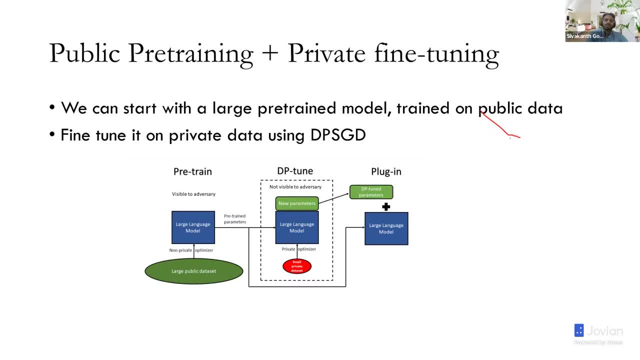 It'll do much better than the public model, because now it knows the patterns of private data but then it learned it in a, in using in a different Private way, but still it's much better than the public model in, you know, in predicting. 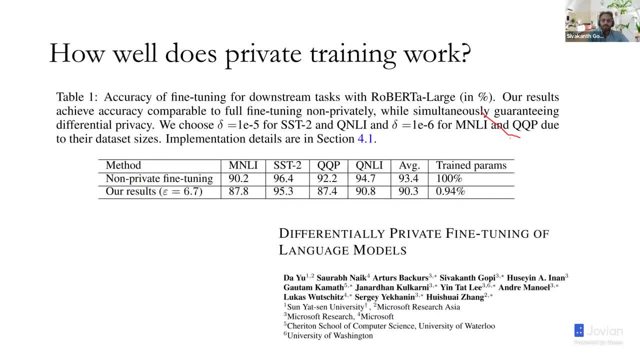 the patterns in your private data. So this is the dominant regime. it's being used right now And you know, here I gave you an example of, like you know, some experiments from my paper we wrote, where we showed that these large language models do really well, even if you.